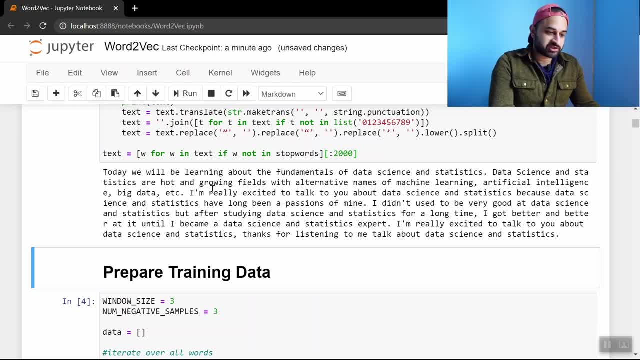 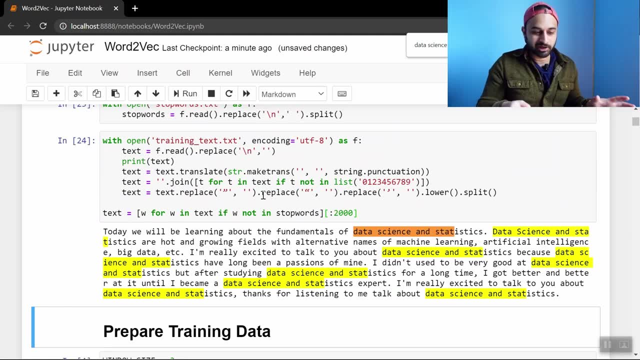 but we'll see what happens when we increase the embedding size. So this text, you can go ahead and read it. It's kind of silly. I basically just put the words data, science and statistics, like many, many times, in here, just to make sure that Word2Vec picks up on all that and puts the words. 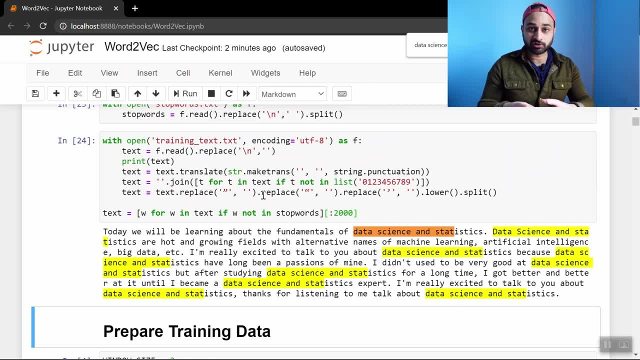 data science and statistics kind of close together in our two-dimensional space at the end of the day, And there's other parts in here that are interesting too, like we have the words machine learning and artificial intelligence, other stuff showing up. So the first thing we do as we talked- 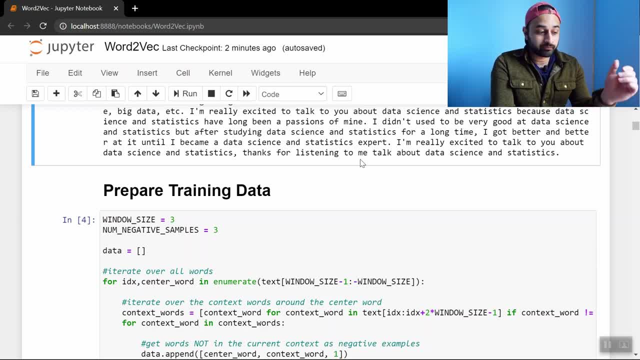 about in the Word2Vec video is we're going to be using Word2Vec. So we're going to be using Word2Vec in this video is that we're going to prepare our training data, And so that kind of consists of three steps. First, we eliminate all the stop words, So there are certain words in here like 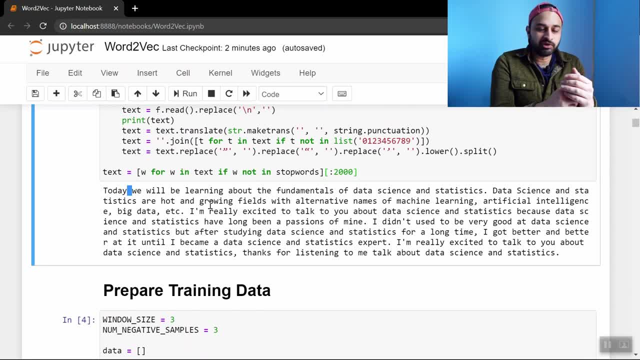 we and the that we'll just get rid of. The next step is we do the skip gram technique, which allows us to construct the data set, And then we introduce negative samples so that it learns what are context words and also what are not context words, And so for this video we picked a window size of 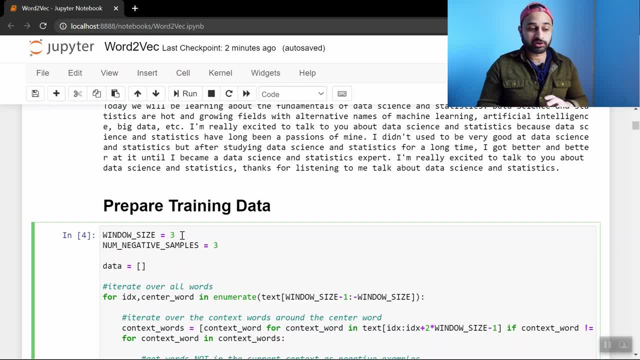 three, so that when we're looking at a main word, we consider the context as three words before and three words after, And the number of negative samples is three, So that for each main word, we include three examples of things that are not in its context And, at the end of the day, we get a data set that looks like this: 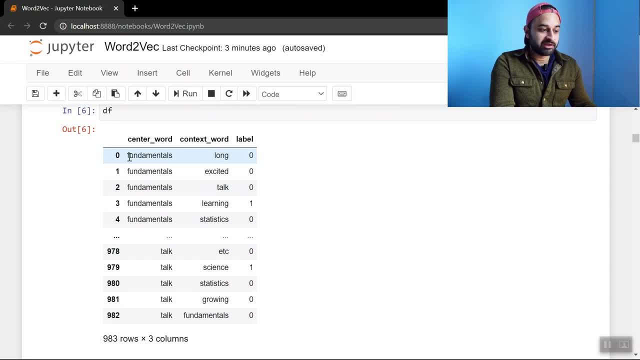 So it's 983 rows, That's how many samples we have, And each one is a central word, a context word, and whether or not those two things actually appear together within the window size in our body of text. So we have ones and zeros in here, which is nice. So next we'll take a look at some of the functions. 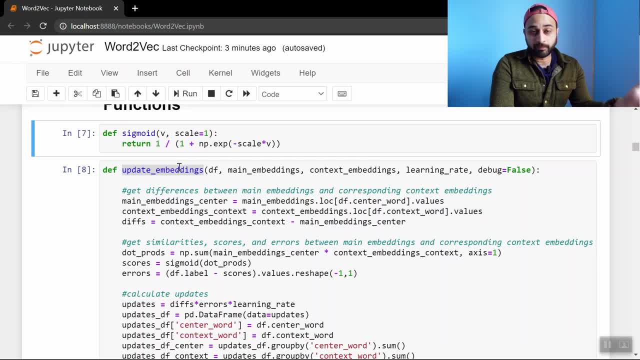 that we're going to use. So this is just a sigmoid function. This function, called update and embeddings, is the one I'll spend the most time on, because that's what's driving this process. This is pretty much one iteration of going through all of the examples in our training data and updating 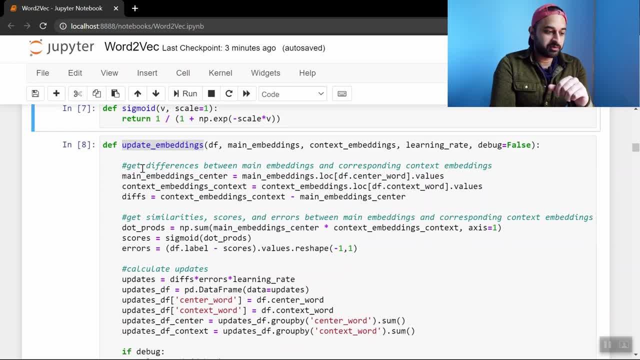 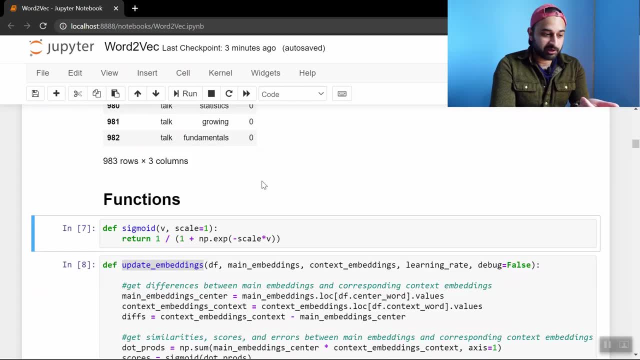 our vectors accordingly. So I've commented as best I can. But the first thing we do is we get the differences between the main embeddings and the corresponding context embeddings, one for one. looking at this data set here. The reason we need to get those differences is because once we figure out the scores and the errors, 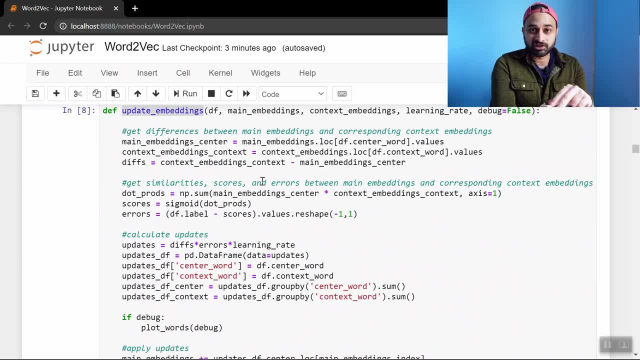 which is the next thing we do. we are going to update each of the main and context vectors in the direction of the data set. So we have a main vector and you have a context vector, and those two things should get closer. Then we use the difference between them to basically bridge that gap a little bit on each iteration. 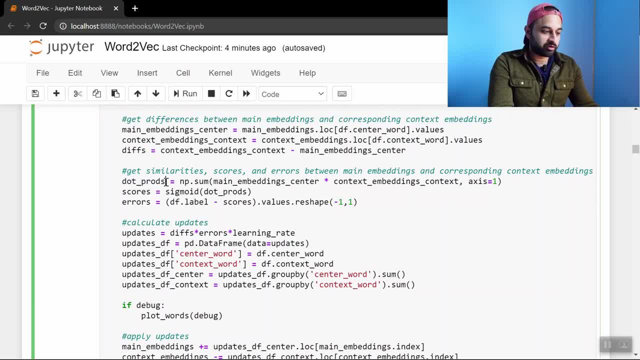 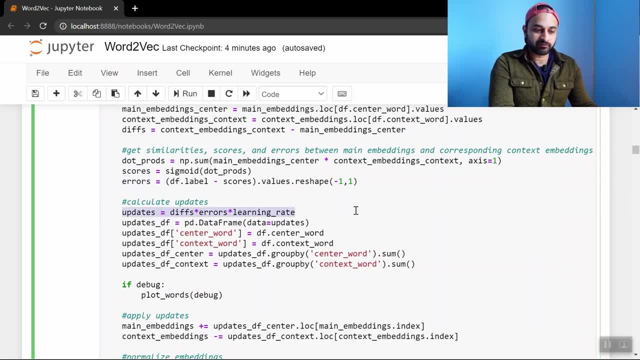 Alright. so the next thing we do is we get the dot products, as we did in the whiteboard video, we get the scores, as we did in the whiteboard video, and we get the errors as well. And this is, honestly, the key line. The rest of this is kind of not as important. 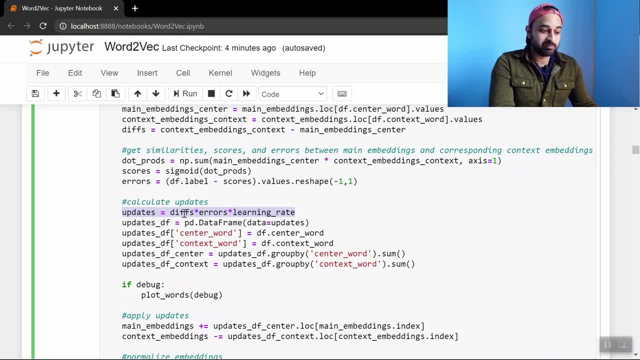 But the key line is that the updates in this current step is the multiplication of the differences, the errors and the learning rate. So let's talk about each one of these and see why this update makes sense. So the differences: what we talked about is the difference between each pair of vectors. 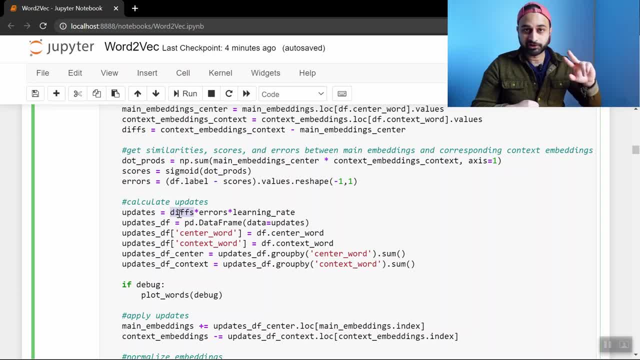 So we want to update in the direction of those differences, to bridge gaps that should be bridged and make gaps wider that should be not close together. The errors is the magnitude of how aggressive we want to be. For example, if we have two vectors like this and the error between them is very large. 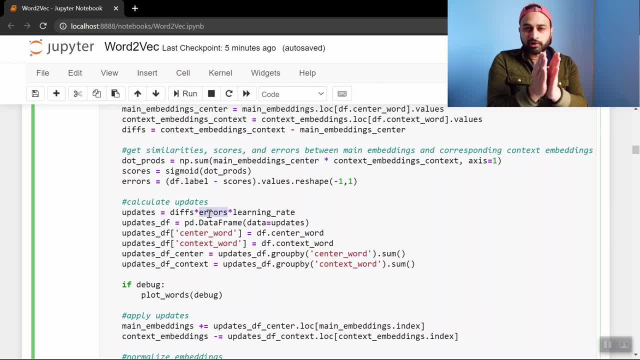 then we want to bring them a lot closer together. If two vectors are already pretty close together, then we want to bring them just a little bit closer. So we're updating proportionally. It's proportional to what the error currently is and the learning rate is just a user-defined parameter. 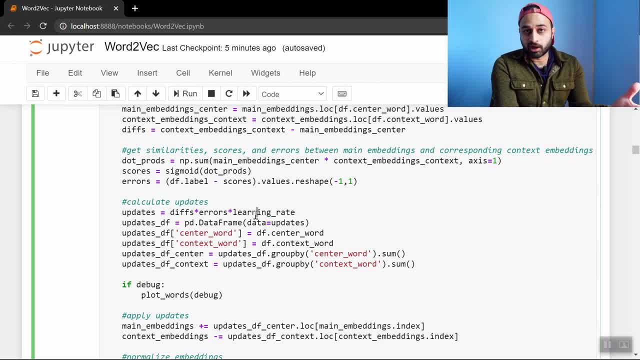 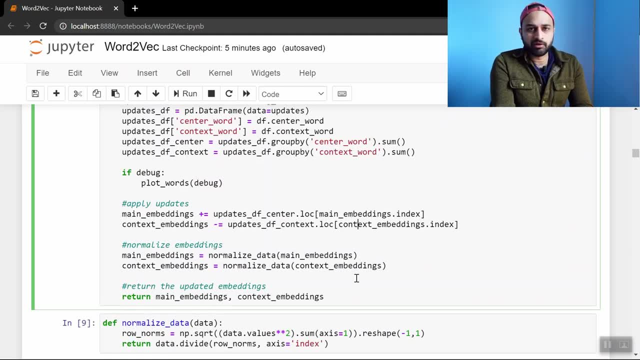 We'll be using 0.1 in this video about how fast you want the algorithm to go, And then the other key line is here, where we actually apply these updates, and that's basically the end of the day. The only other caveat I'll say is that I didn't note this in the whiteboard video. 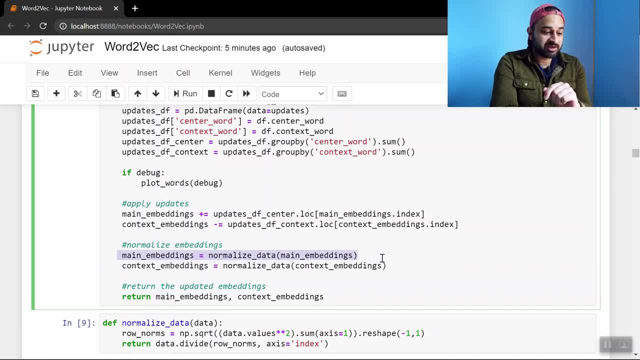 but we are going to be doing this step here where we normalize the embeddings at the end of each loop through all the data. This is to avoid vectors getting way too large. So it's kind of a regularization technique where we bring all the vectors back. 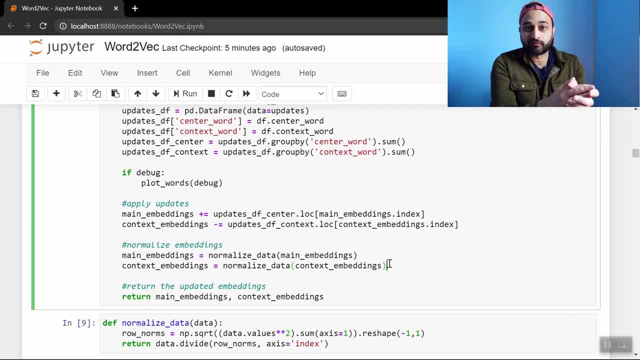 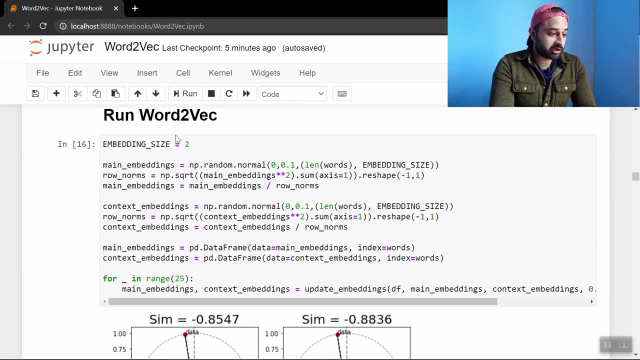 back into the unit sphere, unit circle, unit hypersphere, whatever dimensional space you're currently working in, And that's it. We're ready to just kind of see it at work. So we go ahead and run this driver code here. We're going to start with an embedding size of 2 so we can actually talk about and visualize what's going on a lot easier. 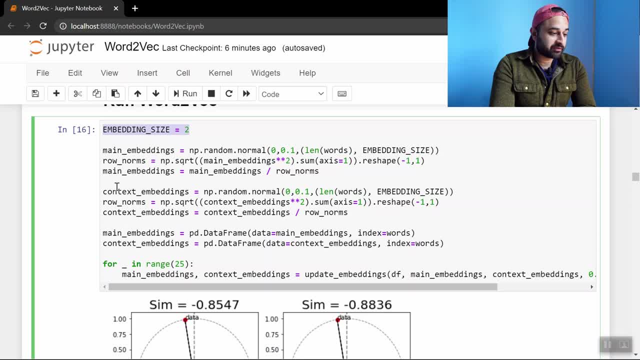 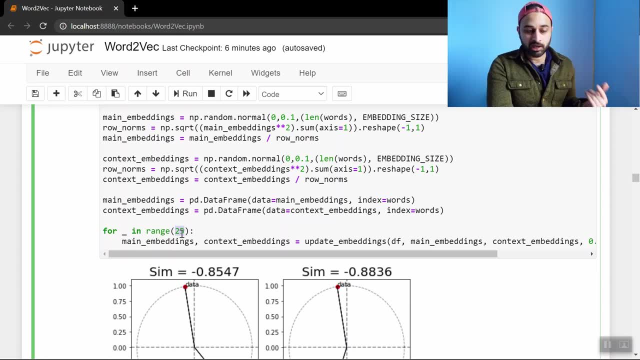 And then we go ahead and randomly initialize the main embeddings and the context embeddings And then we, just 25 times, we're going to run the above function. So we're going to do 25 passes through that data set and on each pass it's going to bring things closer together. 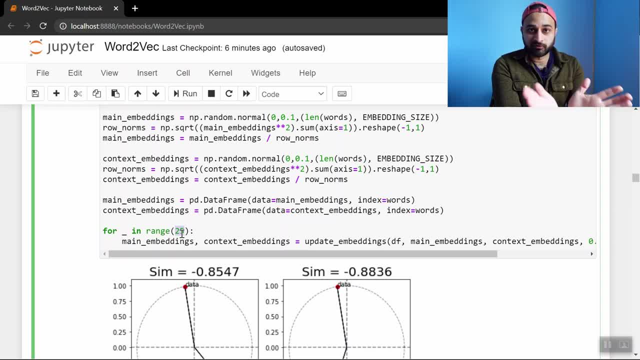 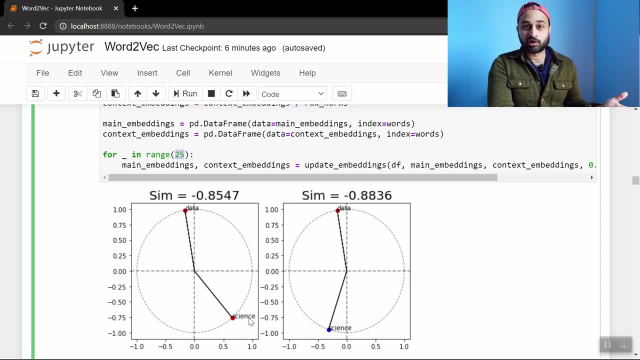 that should be closer together And push things further apart. that should be further apart And we can visualize it here. So I've chosen to lock in on the words data and science And let's kind of treat this as a story and see what happens to them as we go from iteration to iteration. 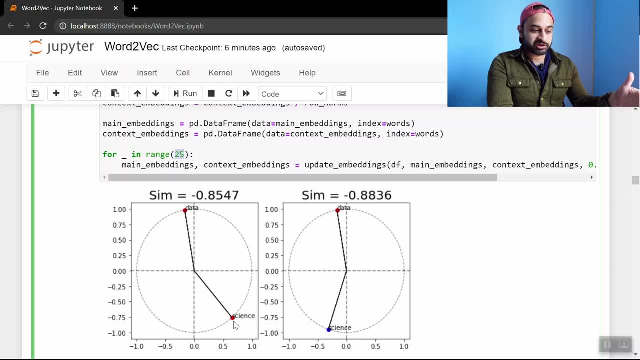 So the left hand plot is the two main vectors for data and science- Remember, the main vectors are the ones that we keep at the end of the day. And the right hand plot- the red one here- is the main vector for data And the blue one here is the context vector for science. 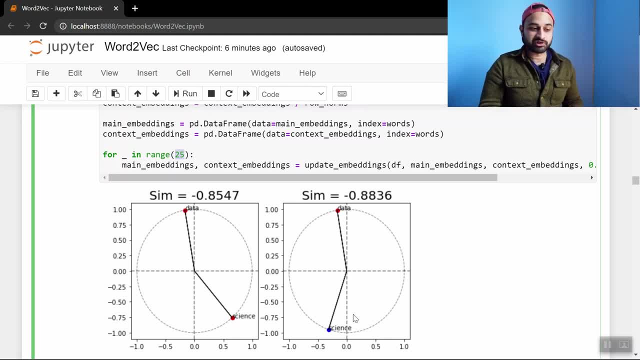 So we can kind of go down this and look at what happens to the main vector And also see what happens to a main vector and a context vector. So initially they're pretty far apart because they've been randomly initialized. So let's scroll down and see what happens to the story. 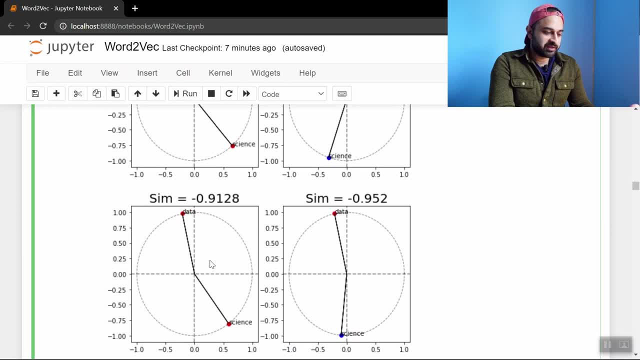 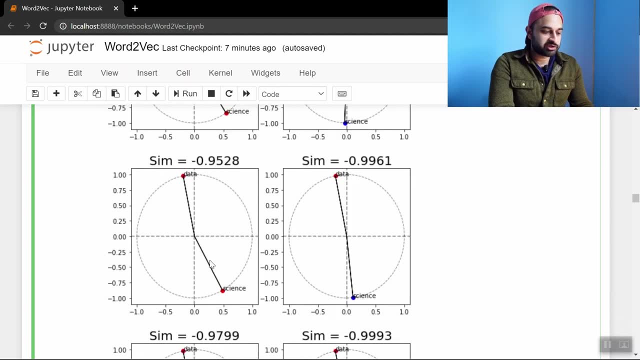 We'll mainly just focus on this left hand plot here So we can see they actually get a little bit further apart. This is while the algorithm is still kind of figuring out what's going on getting past those random values, But pretty soon we see them start getting closer together. 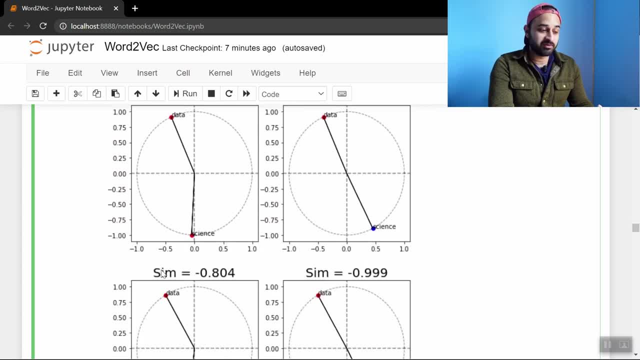 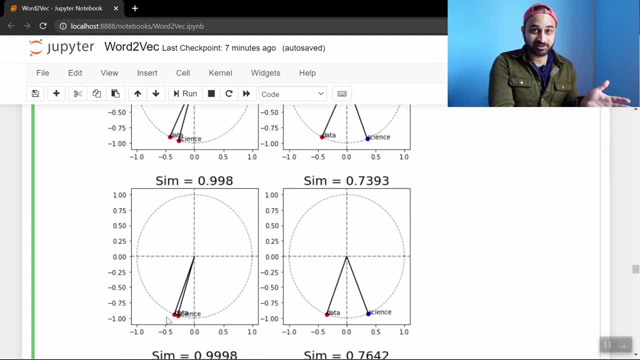 So we see now these similarities, the cosine similarity between them is actually increasing, Increasing, increasing, keeps going. So we see this magical thing happen where they become really close together and we're not even done yet. At the end of the day, it's effectively one. that's the similarity between them. 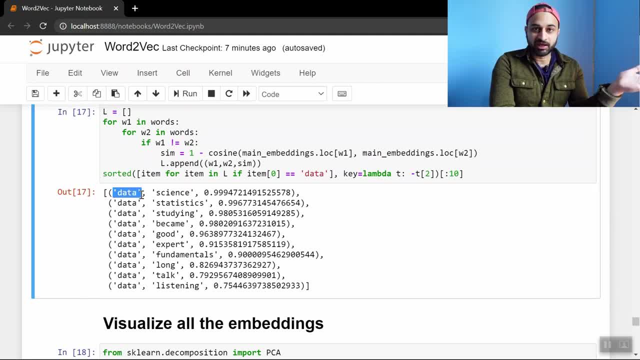 And we can also print out what are the similarities between data and the other words that are in our corpus, And we see that data and science have the highest similarity, followed by data and statistics- also what we would expect, And then some other stuff that happened to be in the neighborhood of data. 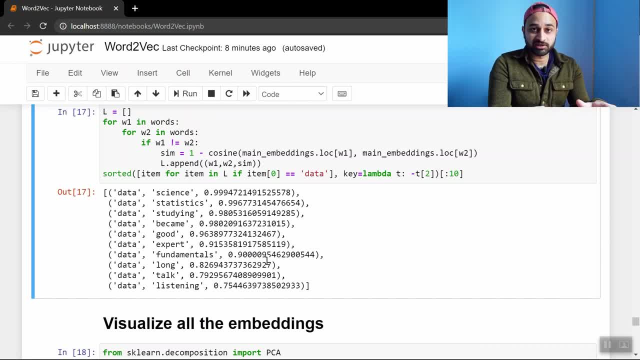 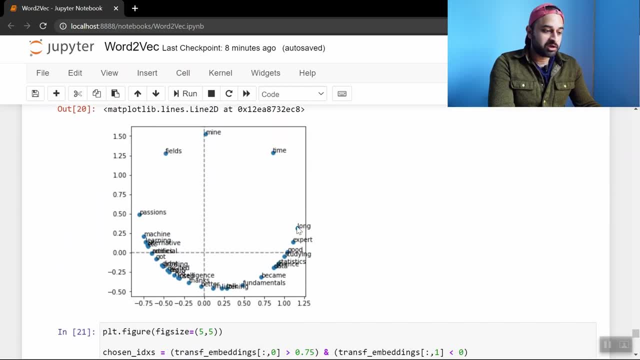 But this is totally what we would expect. We wanted data and science and data and statistics to be very close to each other, And that's exactly what we got. And then, since we have these embeddings, we can just visualize all of them. So these are all of the embeddings. 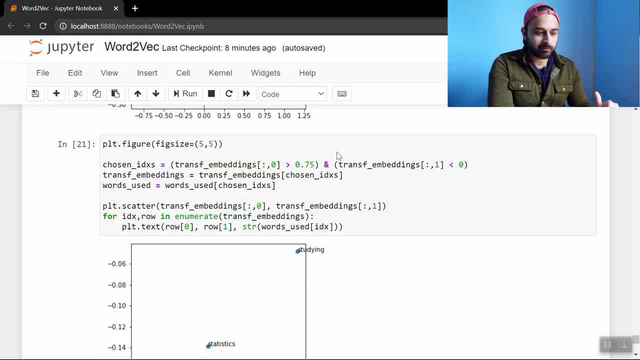 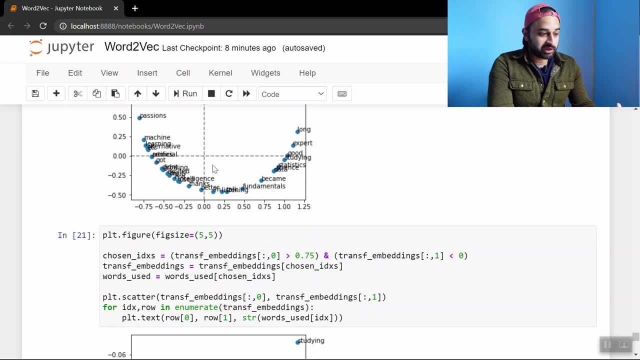 A little bit difficult to look at. so let's zoom in on the bottom right hand corner And we see we have data science statistics all close to each other in this little cloud over here, And then we can look at other interesting things too. 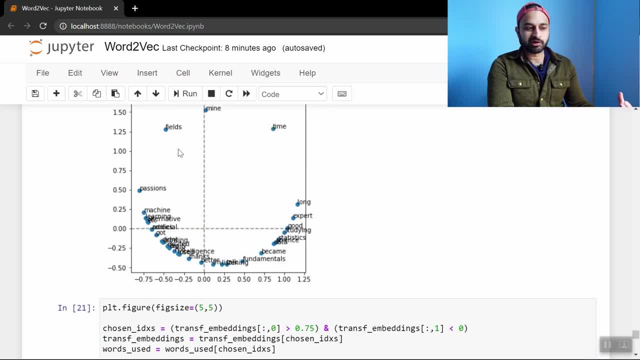 Like we see, we have machine and learning actually showing up together here, So it's doing a lot of the things that we would expect. So now let's increase the embedding size to five, which is still way lower than what it would really be.